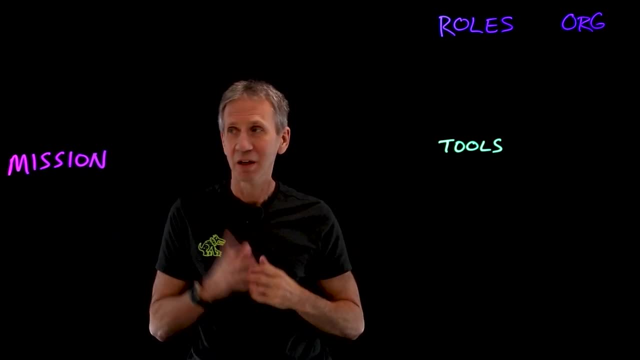 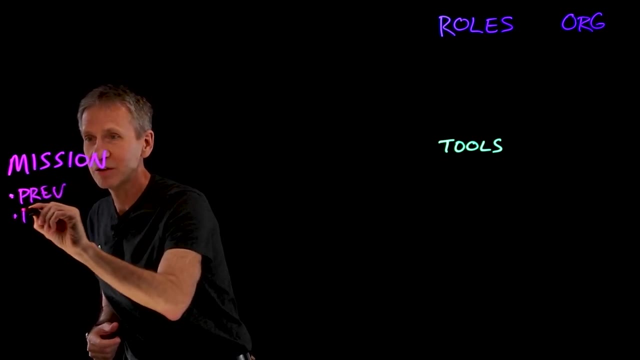 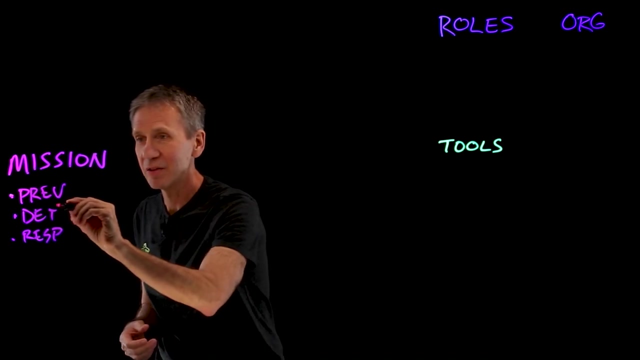 as to how those tools might run in a modern SOC. First of all, the mission. So in security, we're always focused on prevention, detection and response. That's what everything in cybersecurity is about, And the SOC is particularly focused on those last two things. 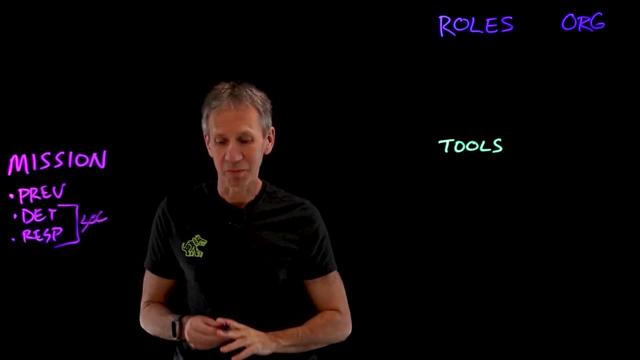 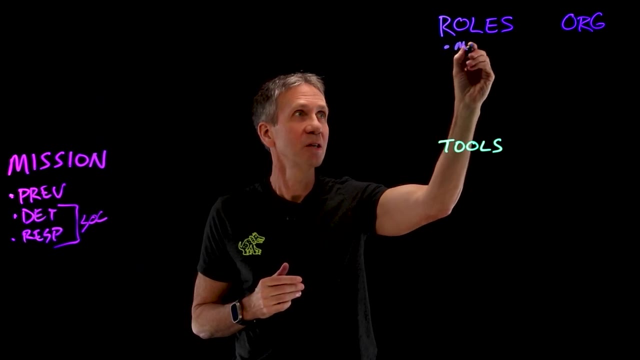 where it's about finding the problems and resolving those problems. Now a little bit about the roles. There's at least four distinct roles I'm going to talk about here. One is the manager of the SOC, who organizes the operations. There is an engineer. 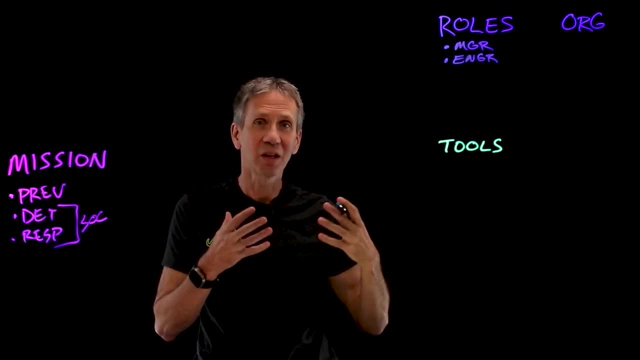 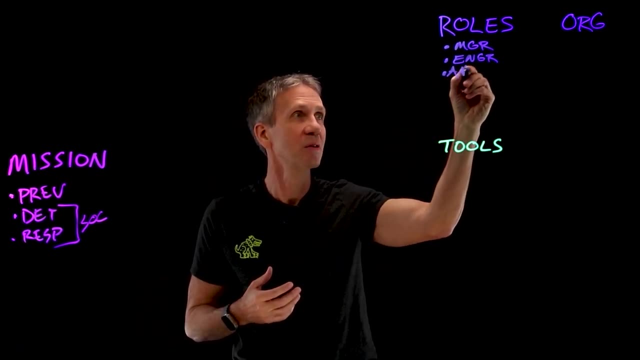 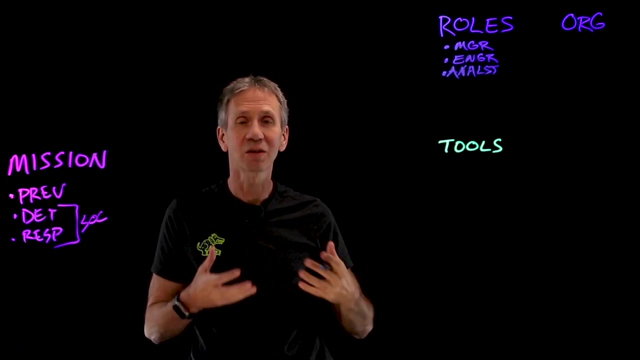 Engineers are the people who are building the SOC itself, as in installing the software, picking the tools, configuring the tools and things of that sort. Then we have an analyst. A SOC analyst is going to be the one who is actually going through the scenarios, feeling the incidents and trying. to discover what was the root cause of those. Oftentimes we have SOC analysts that are organized in different tiers depending on the level of complexity of the problem that they're dealing with, So a Tier 1, Tier 2, Tier 3, where the Tier 1 does the initial fielding of the issues. 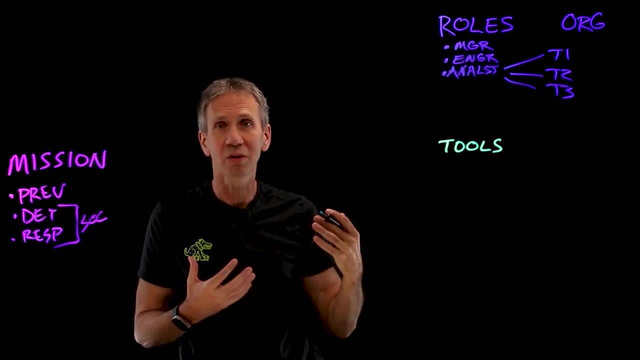 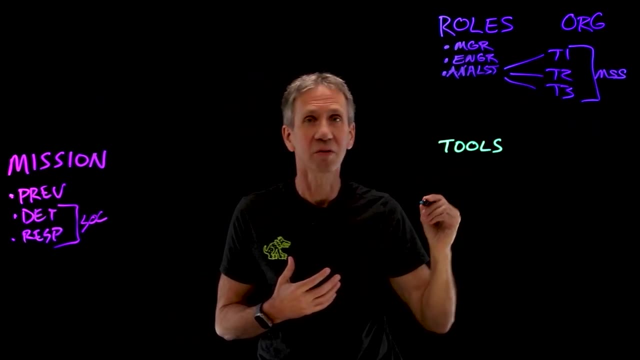 and then, if it needs more deeper investigation, Tier 2 and Tier 3.. Very often these could be done in-house or could be done as part of a managed security service, Or maybe you just have the Tier 1 as the managed security service. 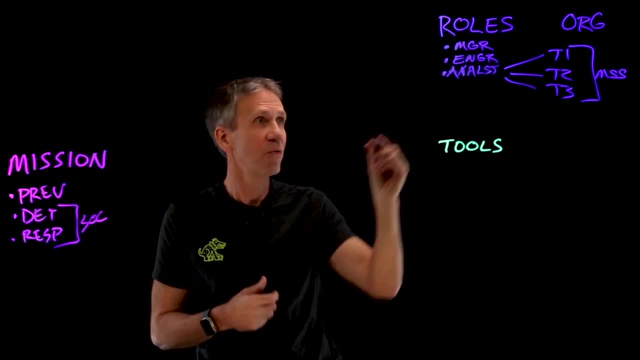 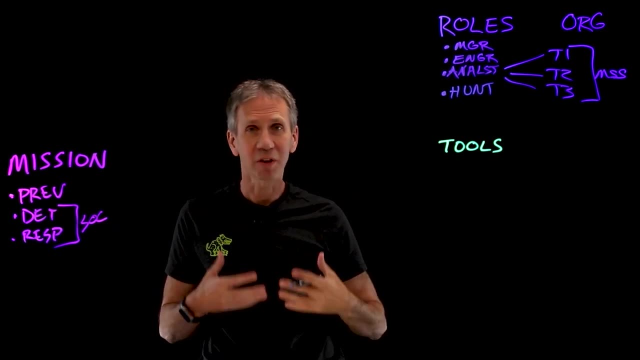 and then your organization does the deeper investigations. The fourth role that I'm going to mention here is a threat hunter, And a threat hunter is someone who is going to come up with a hypothesis and then they're going to go out proactively trying to find where the problem areas might be. 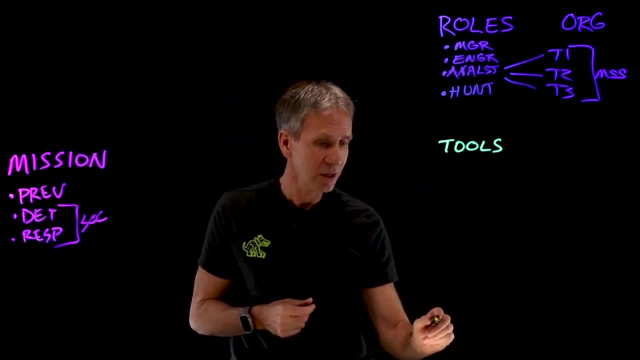 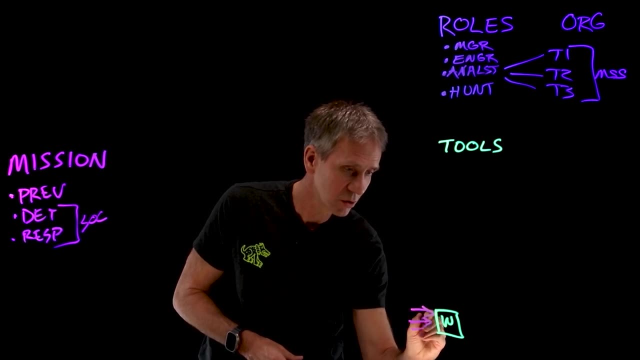 Okay, let's talk about the tools In the tools area. let's take a scenario where we've got a web server And that web server now suddenly starts. It starts getting tons and tons of traffic and it's not good traffic. 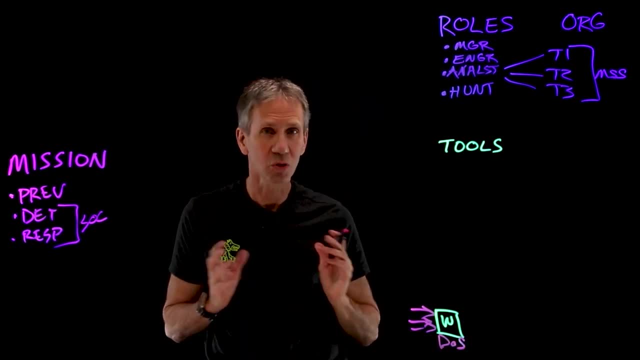 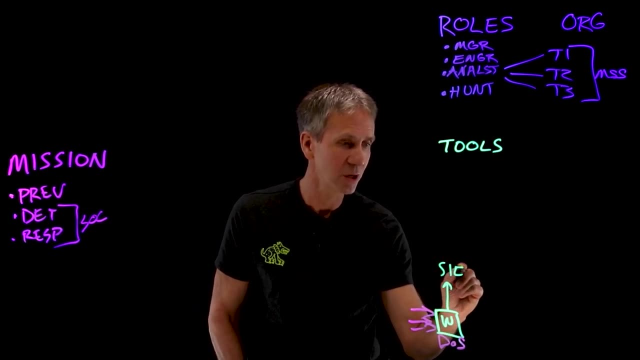 In fact, we're in a denial of service situation, so we're under attack. What could happen in that case is I'm going to take the information from that web server and feed it into something that we call a SIEM, a Security Information and Event Management System. 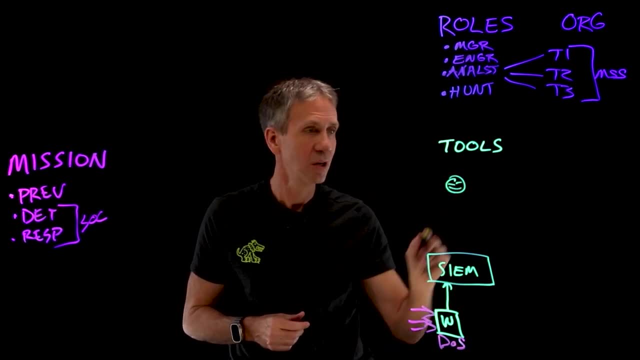 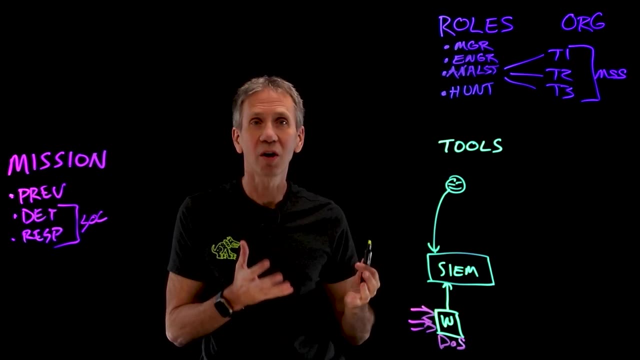 And I'm going to have the cybersecurity analyst here looking into the SIEM and seeing what's happening. They're going to get all of that telemetry. They're going to have the information They need to go off and do an investigation and find out what's going on. 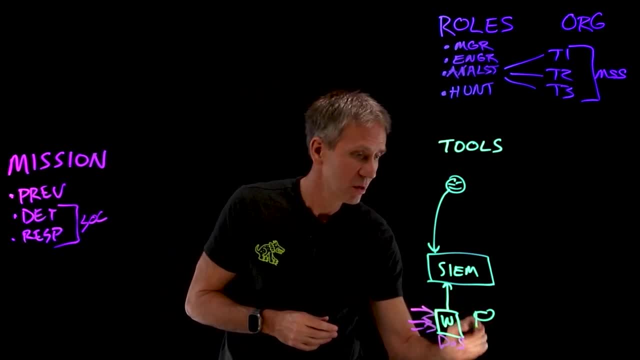 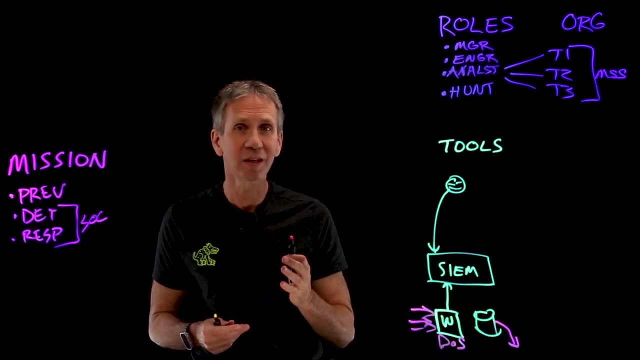 So that's our first scenario. Our second scenario: let's say we have a database with critical information in it and someone is exfiltrating that data, That is, they're taking data out of that system and sending it out into the network. 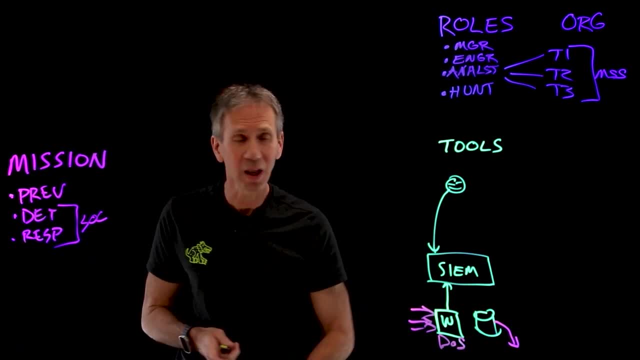 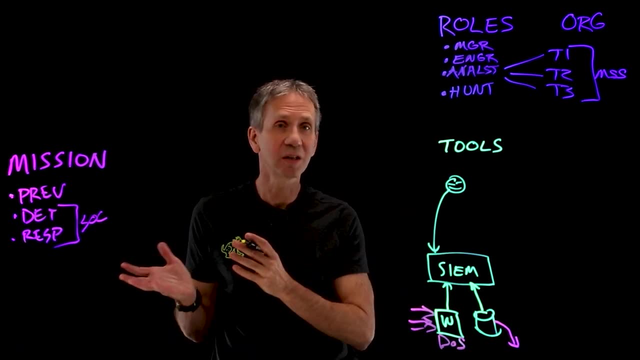 Maybe they're selling it, Who knows what they're doing. But anyway, we would like to be able to detect that there's an anomalous level of activity, either of accessing data or sending data out. And I could use- I could use a technology called a User Behavior Analytics System. 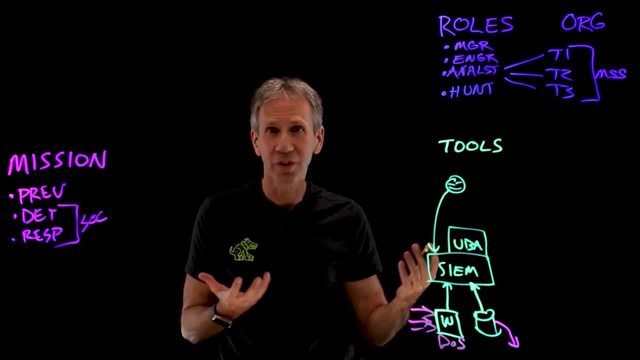 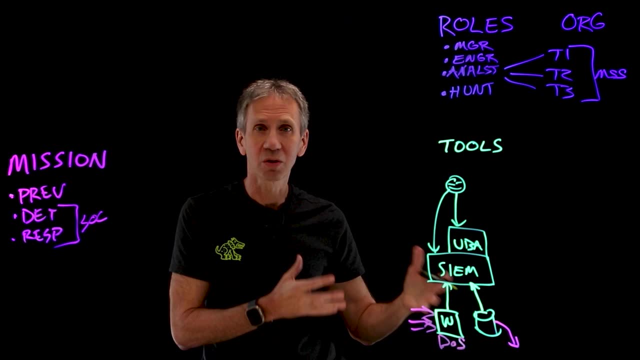 that runs along with the SIEM in order to figure that out, And it would send an alarm up and then this SOC analyst might be able to use that system in order to do further investigations. So that's what an analyst might do in those two cases. 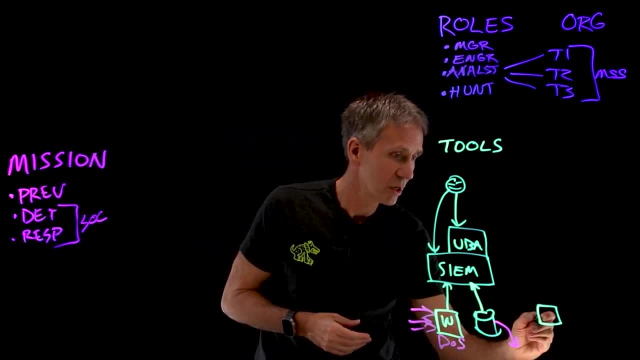 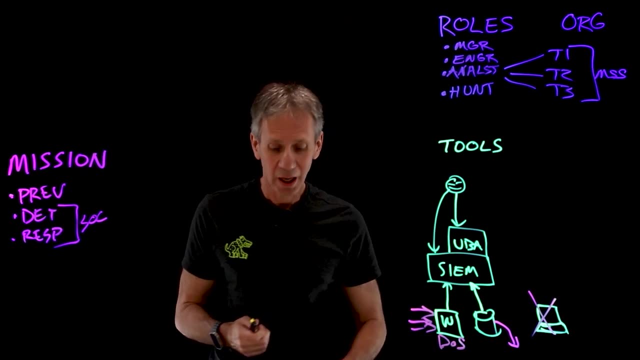 How about let's look at a third case where we have a workstation here and this workstation has been infected by malware, And in fact it's not one, but it's a lot of these workstations that are out here And maybe many of them have been infected and some of them haven't. 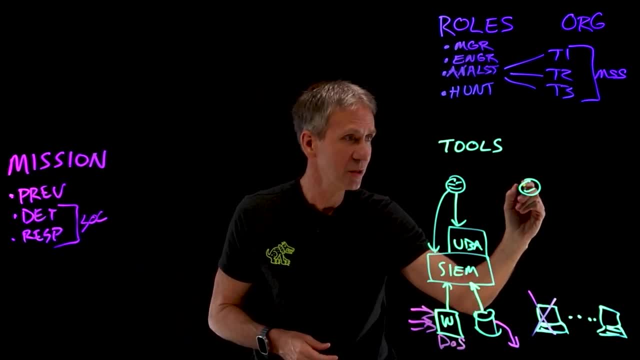 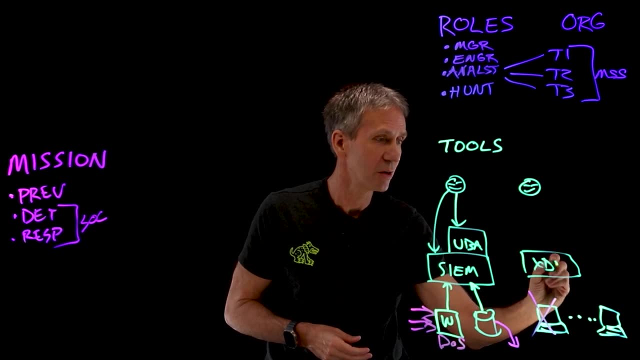 So what would we do? Well, we'd have, in this case, the threat hunter that I just mentioned would be using a platform, and they might use a platform that we call an XDR, an Extended Detection and Response Platform, And what that tool does is it allows us to query information in what we call a federated search. 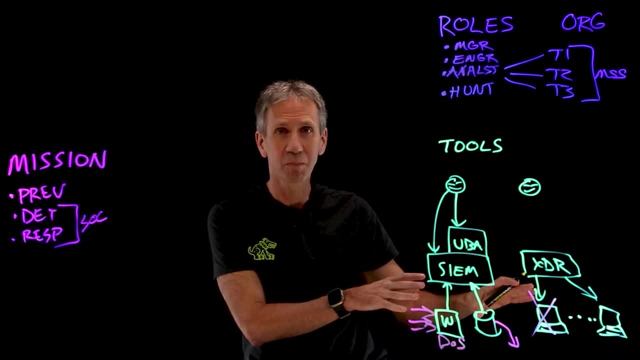 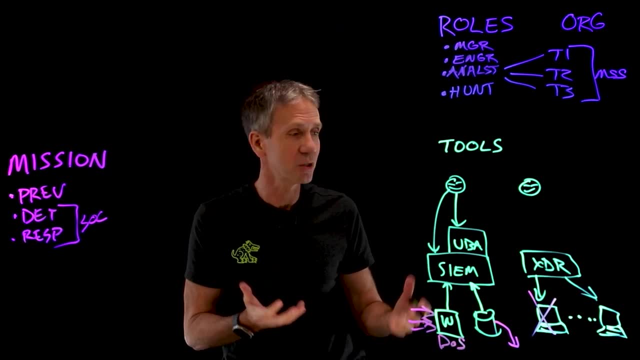 Pull this information. This is the information that I need to find out what the threat hunter is doing, And I can do that information just when I need it. So I leave the information in place until I need it, Where the SIEM is bringing all the information up and fetching that in advance and acting as an alarm system. 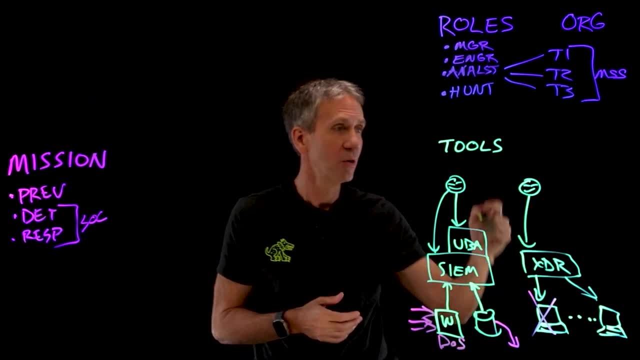 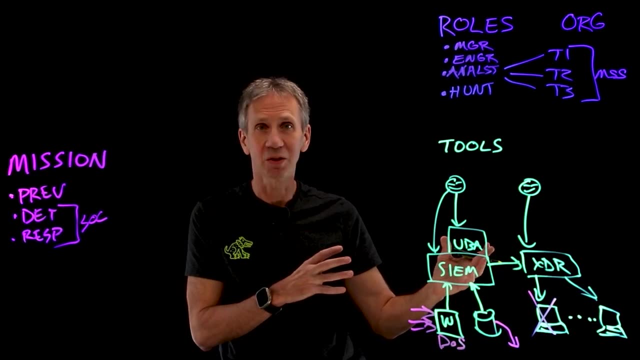 this is more of a go out and look through the information and figure out what I want to do. So our threat hunter uses the XDR system to do that. Now we would also have the ability to have linkages between these systems. That would also be very important. 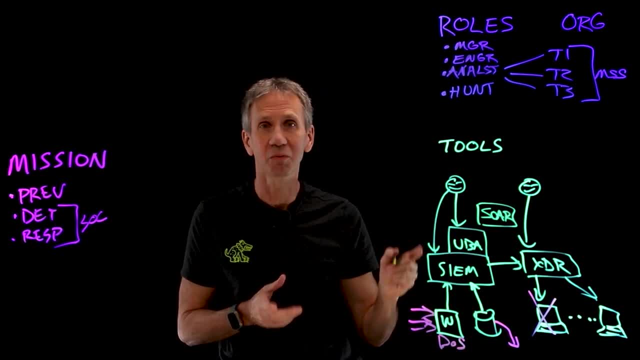 And then ultimately leverage a system called a SOAR, which is a demonstration automation and response system that either of these people could use in order to go out and guide their activities, orchestrate the response, use a dynamic playbook, open a case.